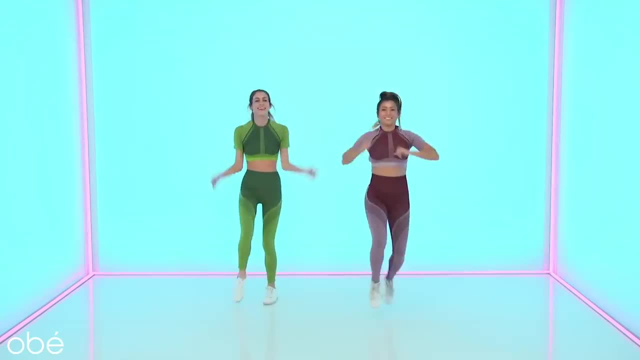 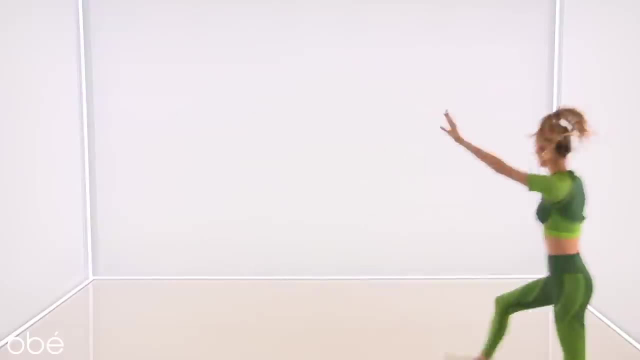 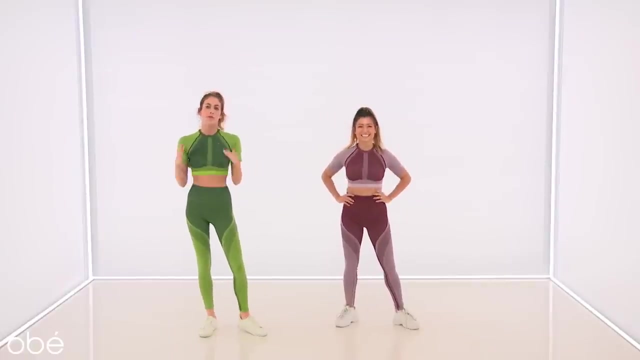 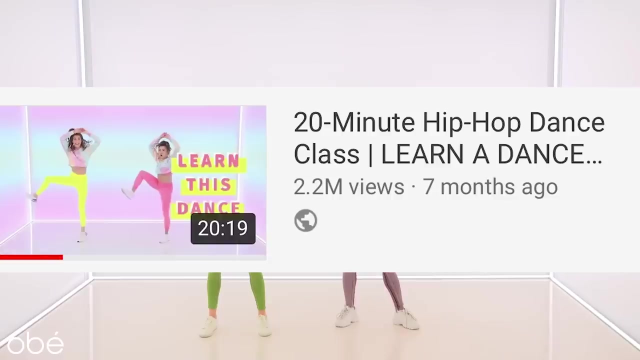 Hey YouTube, welcome back. It's Lucy Fink. I'm here again with Sarah Burke at Obey Fitness and we are back for round two of those dance videos that you seem to love so much. So I posted one a few months back and it is in the millions of views by now. Crazy, So this one's a little bit. 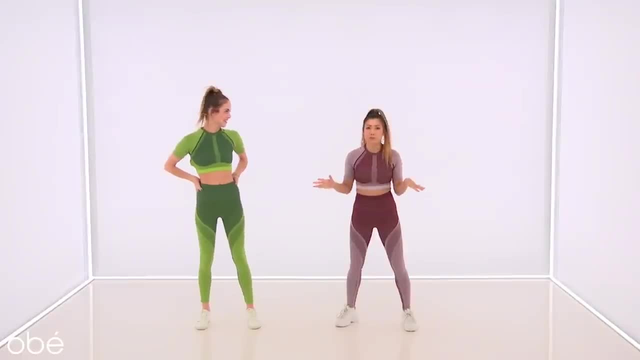 harder than last time, but that's okay. As always, if you feel like we're moving too fast, just rewind until you feel comfortable. Don't forget: if you do this dance and you love it, be sure to record a video of yourself doing it and then tag both of us on Instagram. I will put our handles right. 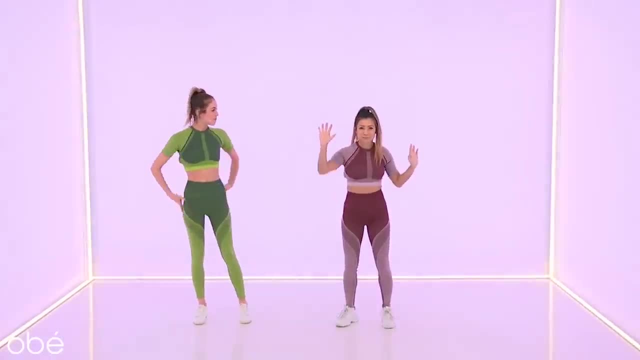 above. So I'm going to teach you two, eight by eight. Use this as your mirror, Left hand, right hand. We got you, So I'm going to show it to you. So you give me one, two, three, four, five and a. 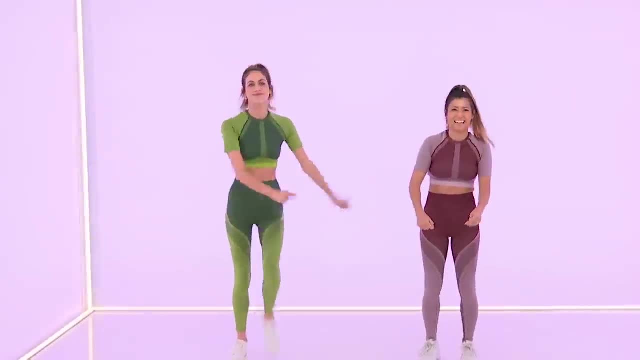 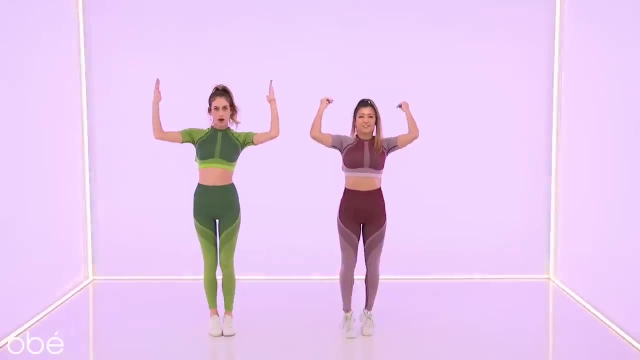 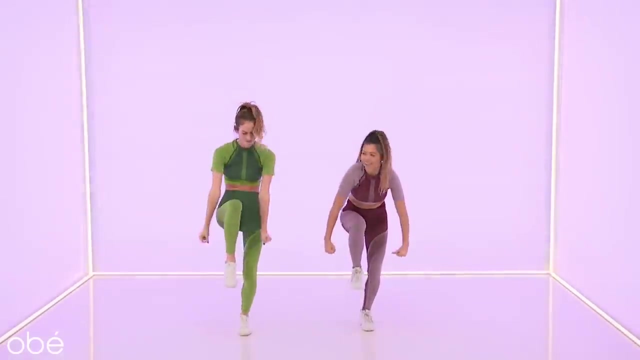 six and a seven and an eight. Go, You're going to step forward with your left and cross your hands. Then step together and give me a touchdown and then crack it over that left, because it's nutcracker season. To the side, Bring them up, Crack her down. Step forward with your left. Five, six, seven. 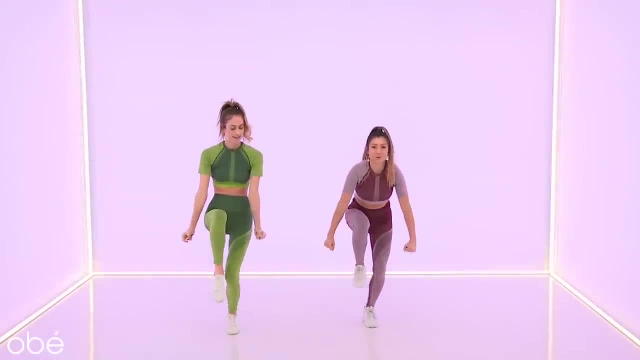 eight. Give me one, two, three. Now which leg is up? This is my left leg, Amazing. Step across with it. Five, six, seven. From the top step it: One, two, three, four. Sink that up. Five, six. 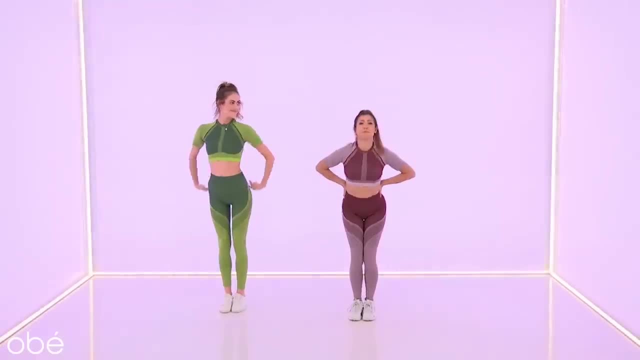 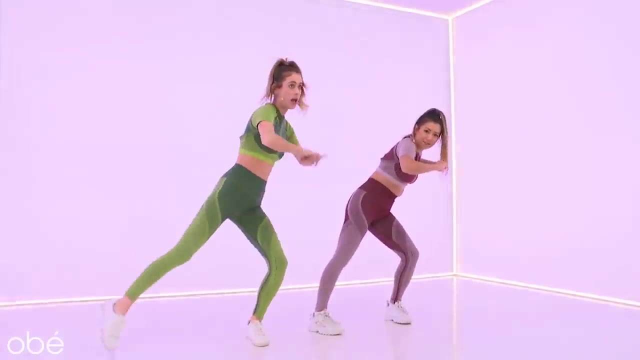 seven, eight And one, two, three, four. One more time, and then let's move on: Five, six, seven, eight And one, two, three, four. From here you're going to take it out Five, Switch it A six, And 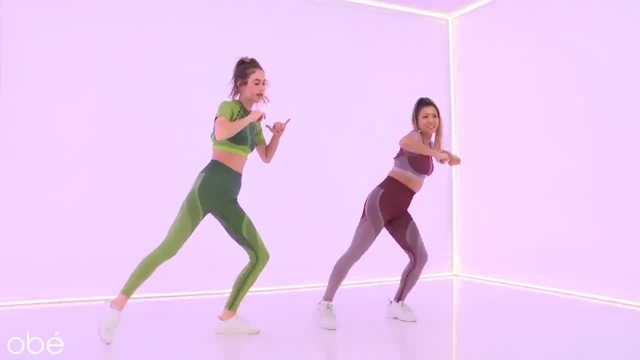 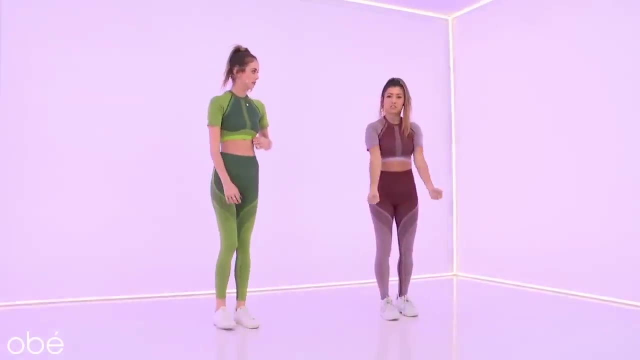 a seven, Double it up. That's one of my favorite moves. And eight: I always think of Backstreet Boys when I do this. Yeah, It's very Backstreet Boys, Backstreet's back. All right, Make sure that you're pulling up versus working those biceps. Yeah, So you just went four. You're going to cross. 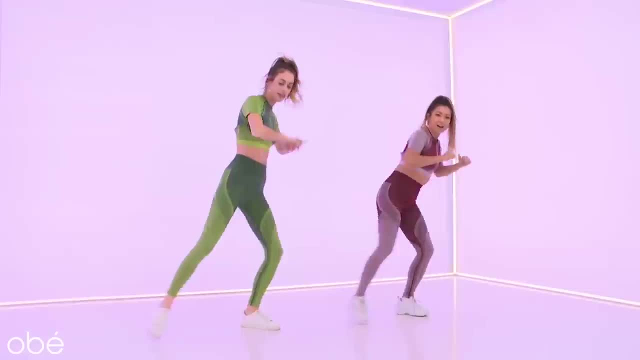 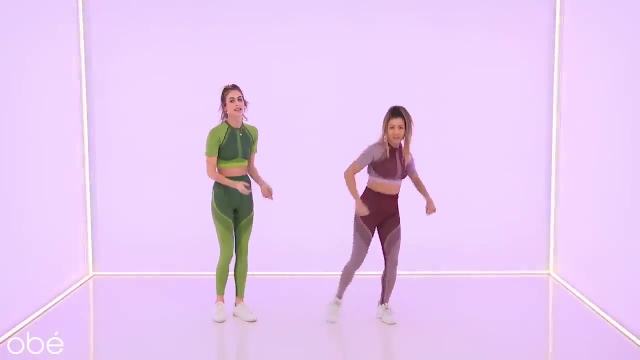 it out: Five a six, four, five, six, seven, eight, One, two, three, four, five, six, seven, eight. And are you breathing? I always forget to breathe, So you got to go. I think the microphone guy is. 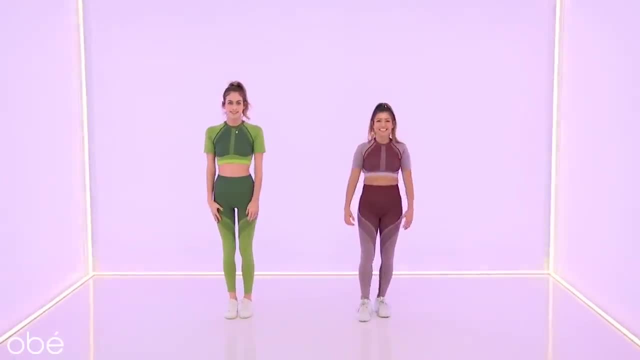 going to be upset From the top, From this thing: Five, six, seven, eight. Step it One, two, three, cross it Four out: Five a six, a seven, a eight. How was that So good, Great, Do it again. 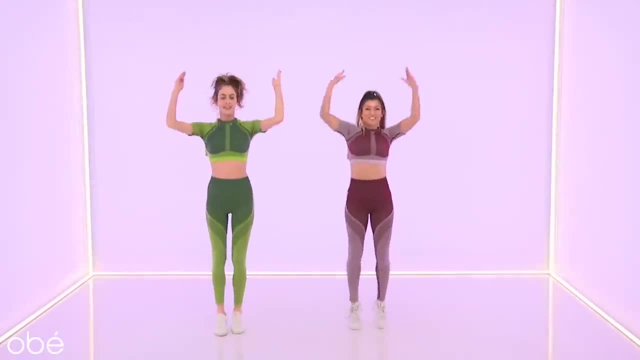 Five, six, seven, eight. Cross them One, two, crack it Three over four out Five a six, a seven, a eight. Okay, Now we do it faster, Okay, Okay, Five, six, seven, eight And one. 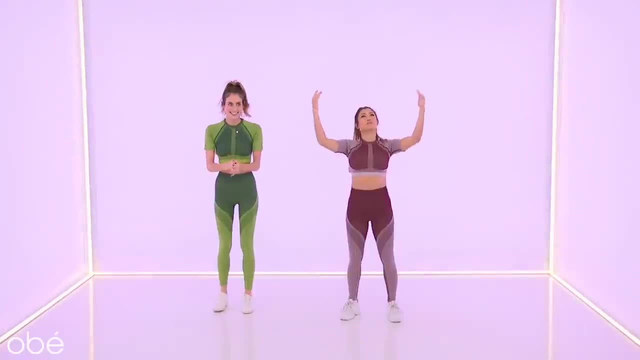 two, three over four, and a five and a six and a seven and a eight. If we get the music, gods to please play the music for us. You're starting to hear that beat. You can move before I count you. 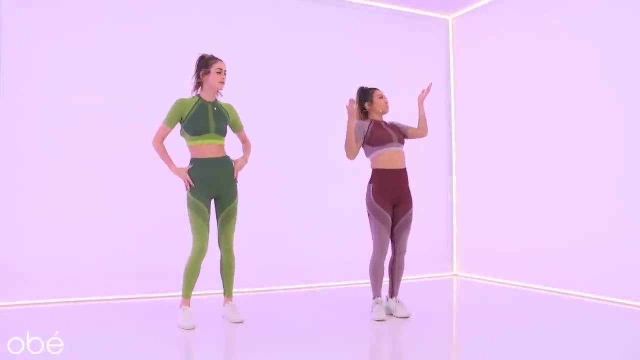 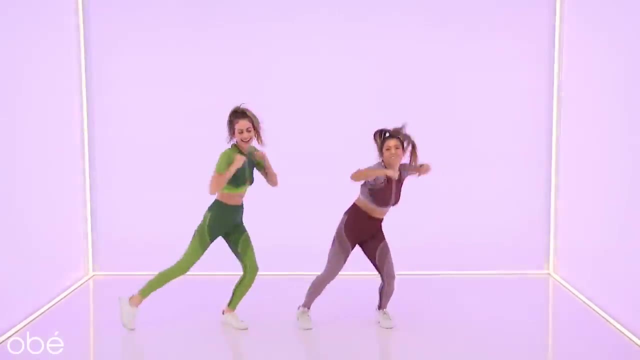 in. I'll always count you in: One, two, three, four, five, six, two, one, two, three, four, five and six and seven, eight. Again, Ready, Get that music going. Oh, you're so ready. Five, six, seven, eight. 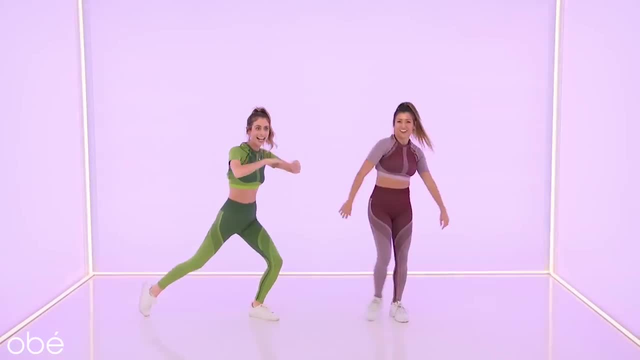 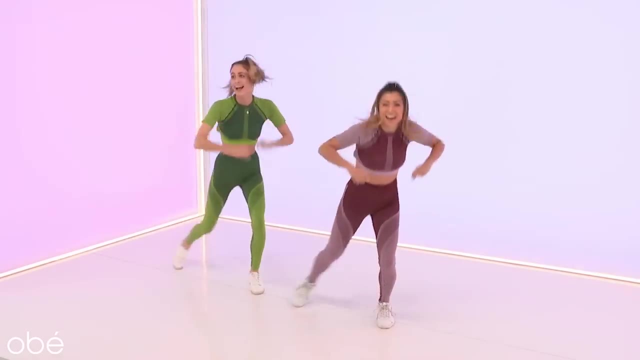 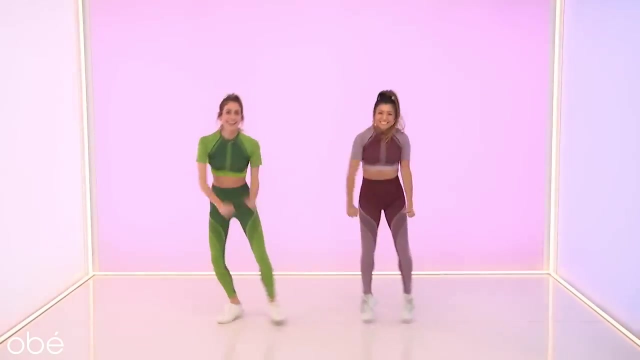 One, two, three, four, five, six, step it. And one, two and out and out and again Ready. Five, six, seven, Okay, And let's keep going. Seven, eight, Oh. let me show you first How. 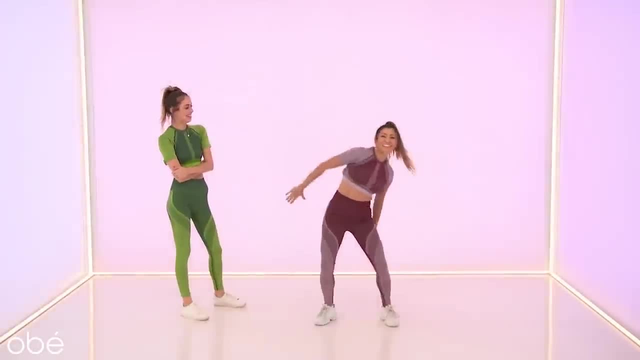 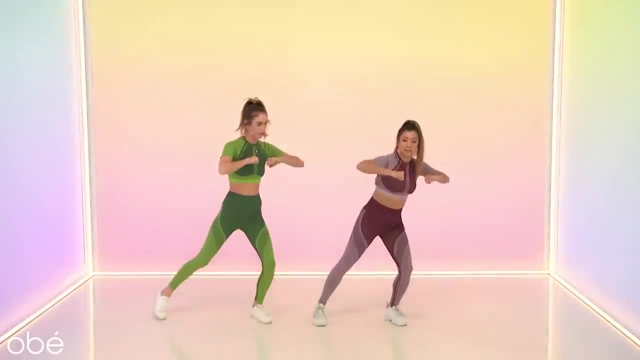 about that. That's a good idea. I'll watch from here. Give me one, two, three, four and five and six and seven, eight. So you just went: seven and eight. You're going to push it over. sweep it One step together. Two, jump it out Three. 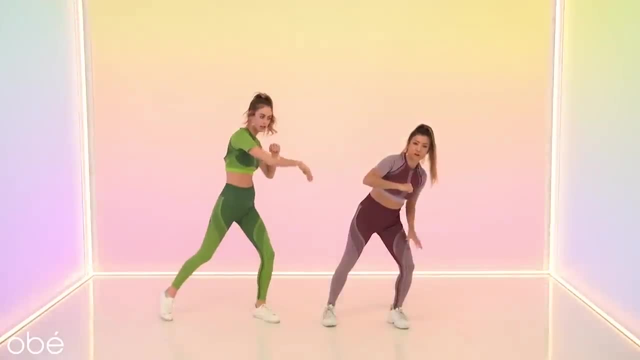 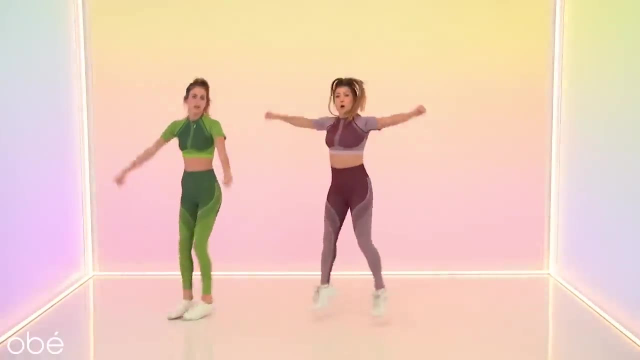 four, ooh, seven, eight. Your weight's already on your right, so you got to go left. Sweep it left, Step together. When you jump out, hit that chest. Boom, One, two, boom. That's the music gods. 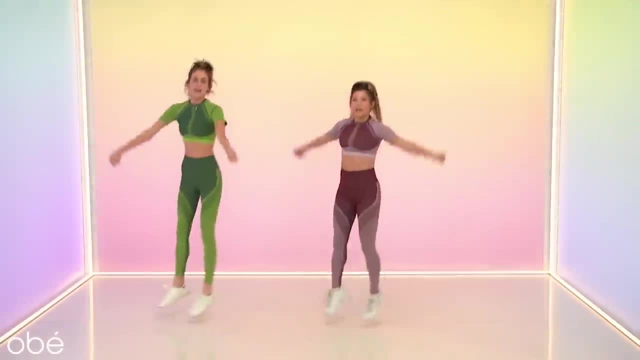 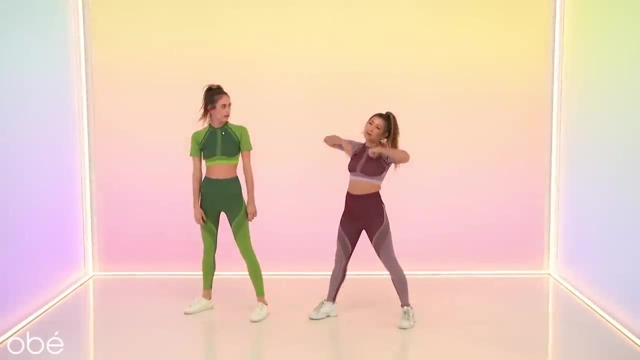 Got it, Five, six, seven, eight and one together. and boom, Oh, five, six and a, seven, eight and one together, boom it. That's it And you're welcome. You get two counts to enjoy this. 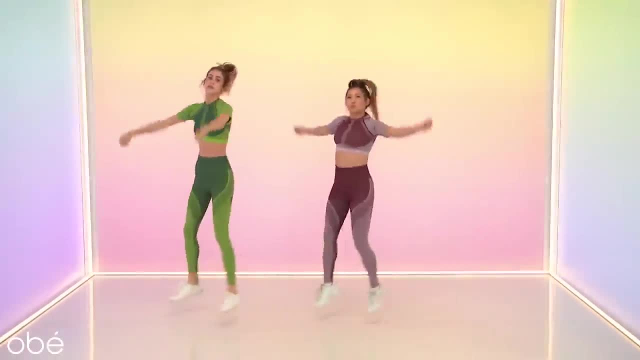 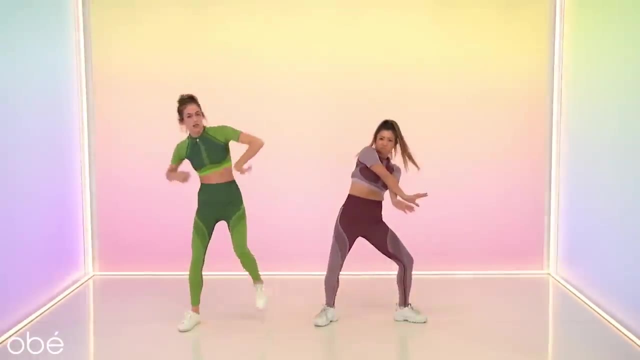 Let's do it: Five, six and a, seven, eight and one, two, three, four. From here you're already facing the left, so let's step there. Another side, Very Dragon Ball Z. Oh, it's very Dragon Ball Z, Dragon Ball. Yes, Should we keep our wrists together? 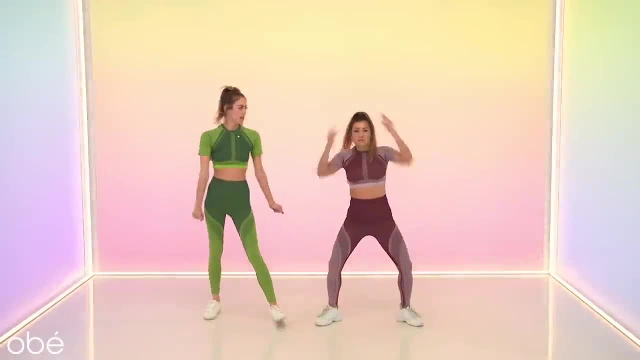 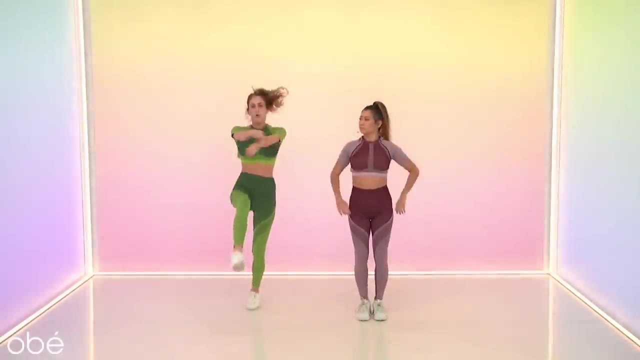 Let's keep our wrists together somewhat, Otherwise it looks like this: A dragon ball On the Z. you're going to jump back on your right, kick your left. Cute, I call this Slice the Pizza. Love it. It's a nice horizontal slice of pizza as you kick it. 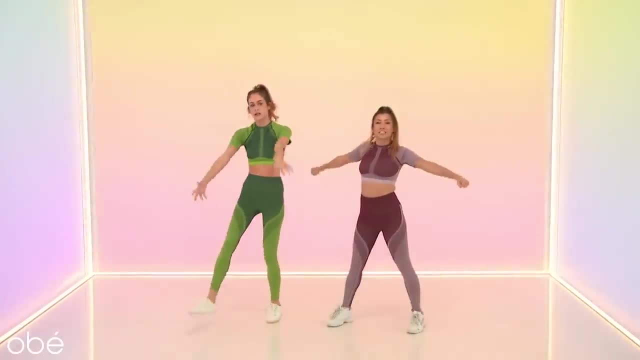 You just went. one, two, three, four. you're going to step on your left. Fifth, six, slice that pizza. seven together, eight. You are jumping backwards on that. Yes, I should see hot, hot, take it back. 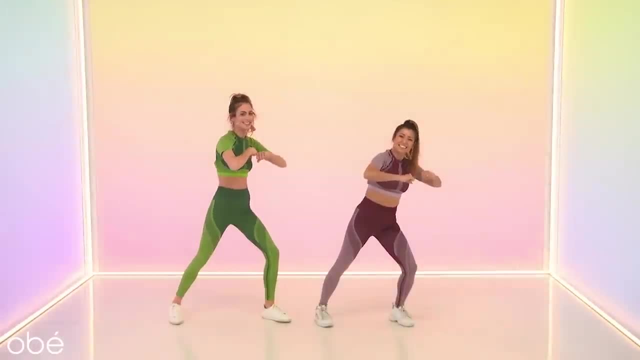 Hot, hot, take it back. Five, six, seven, swipe it out. One, two and a three. step it out in a dragon ball Z. Five, six, seven, swipe it out. And one, two, three and a five, six, seven, eight. 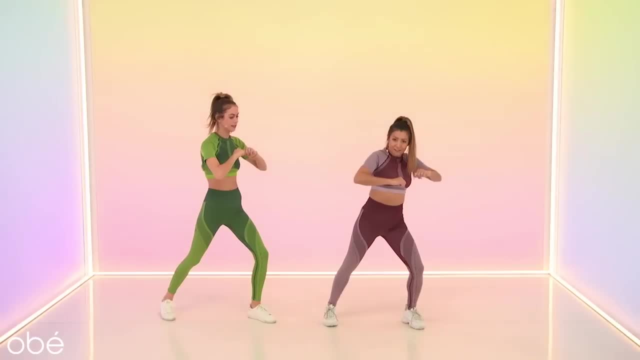 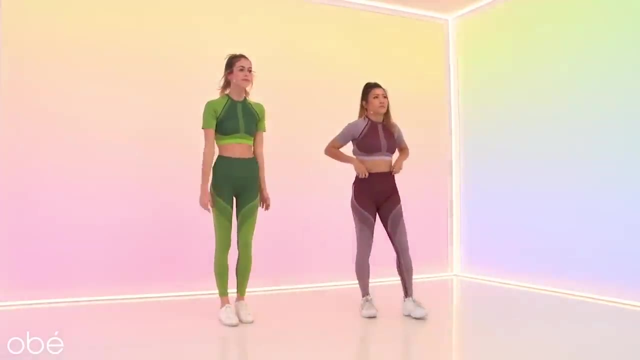 What pizza are you going to order at home now? Pepperoni with olives. Five, six, seven, eight And one, two, three, four and five and six and seven, eight Top. Okay, if we're going to go from the top, got to pull her up. 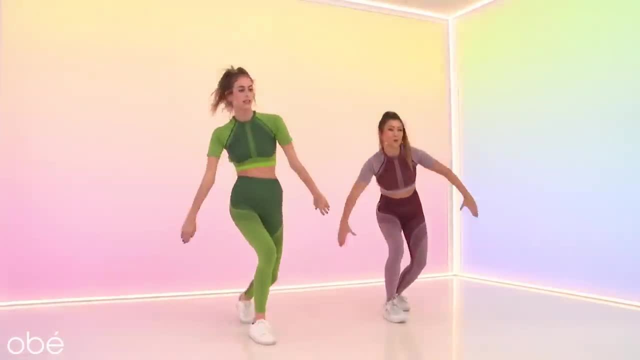 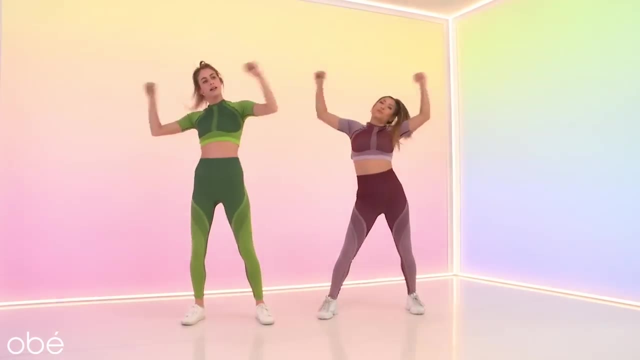 Okay, five, six, seven. left foot goes One, two, three, cross it four out five, a six. new part: Swipe it one, two, three, step it out with a dragon ball Z. 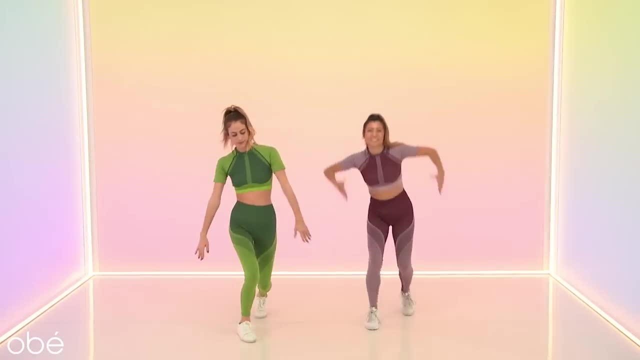 Together Five, six, seven, eight. left one together and crack it, cross out out new part. Swipe it one, two and a three, four. step it five, six, seven, eight. 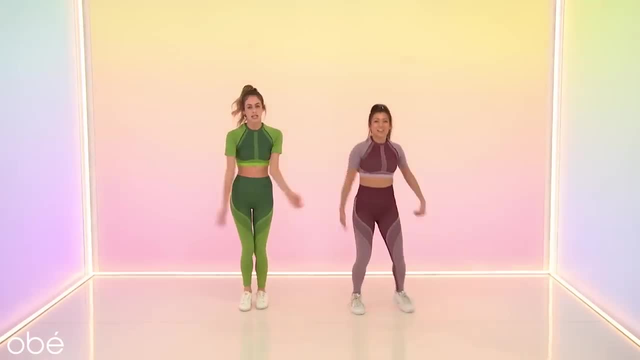 Five, six, Five, six, seven, eight and one, two, three, four, five and a, six and a seven, eight, One, two, three, four, five and six, and we can do it again. 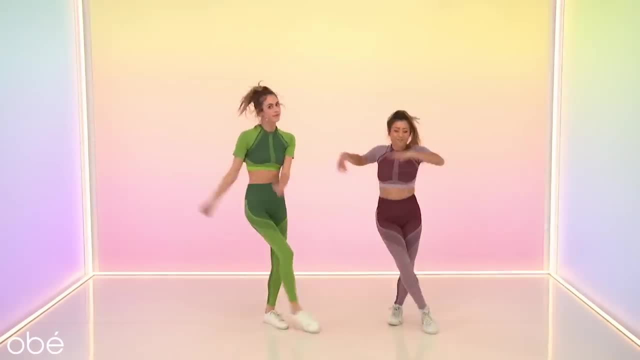 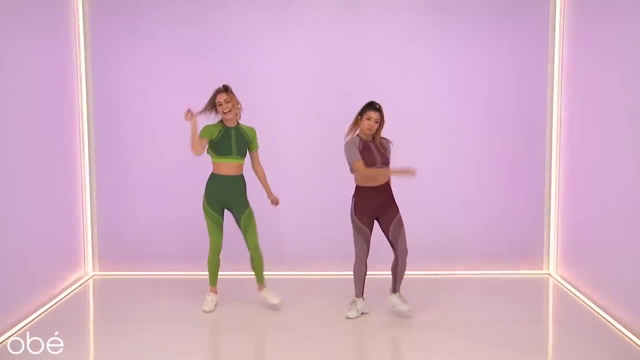 Five, six, seven, top One, two, three, four, five and a six and a seven, eight. Swipe one, two, three, four, step five and six and pizza, Oh girl, you bad. 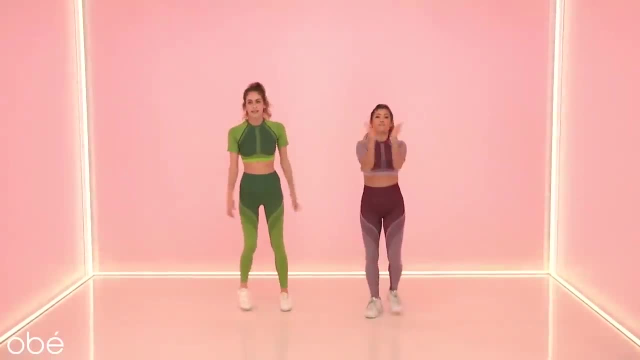 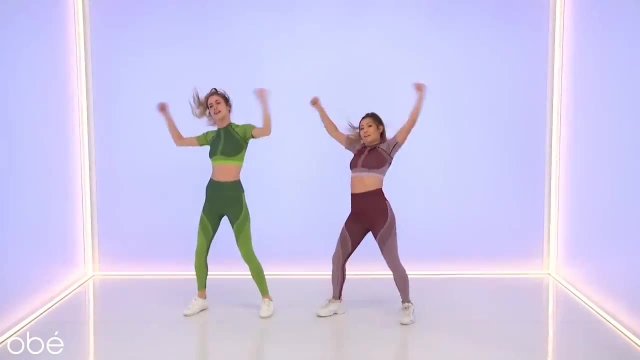 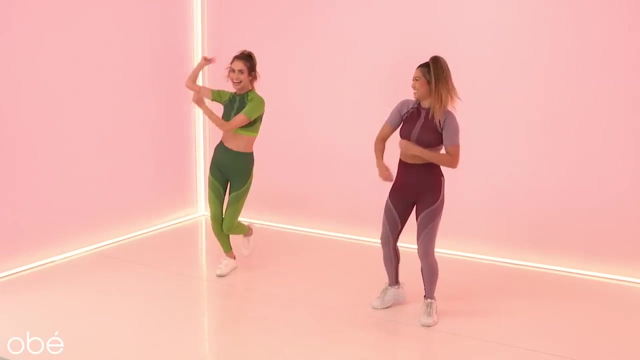 She hit the track and she shut it down. One, two, three, four, five, six. step it drop. You're the best, Swipe it out. Pizza Massage: the beat Eight, Six, Seven, Eight And seven. 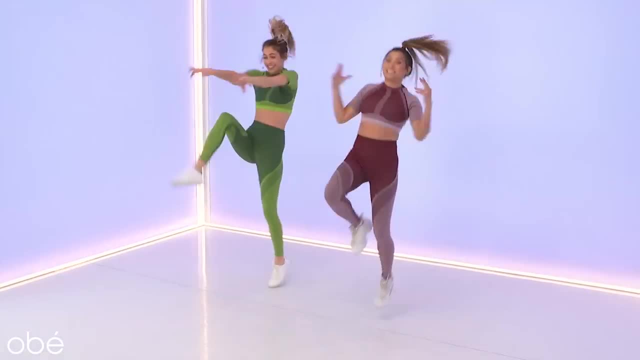 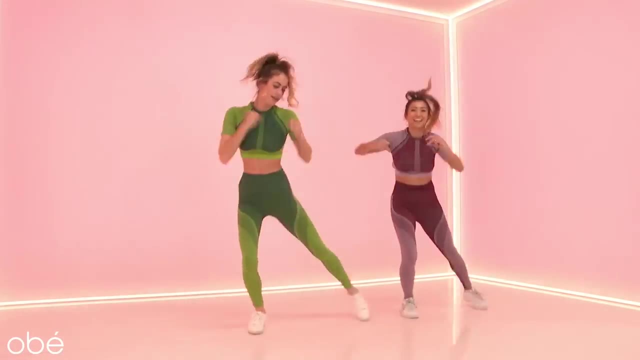 Eight And one, Two, Three, Four And five And six And seven. Eight, One, Two, Three, Four, Five, Six And out And out And double up Swipe, Step it Pizza. 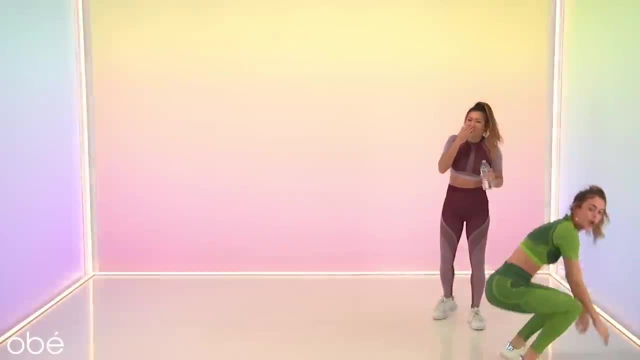 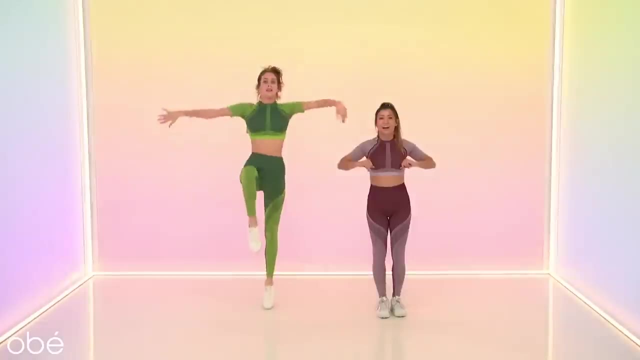 We did two eights. You want some water? Yeah, It's very important to stay hydrated. I'm back. What is this box made of? Just like Backstreet Boys Fabric. I'm gonna keep going. okay, Again, remember, if we're moving too fast, just rewind. 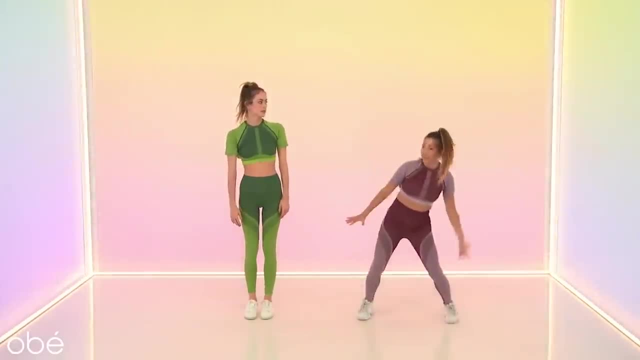 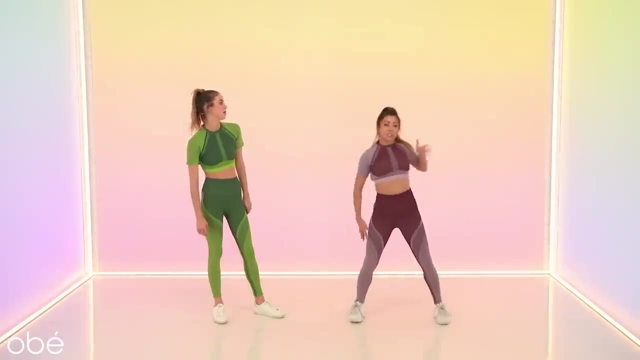 So you just went pizza. You're gonna go one, Two, Three, Four, Kick it Five, Six, Back Seven, Front Eight. Whoa, Scrape it, Scrape it, Scrape it To the Kick it, Kick it. 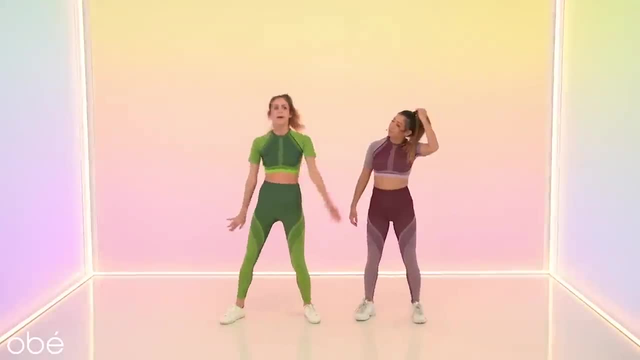 Back Front. Scrape it, Yes, Scrape it, Yes, Scrape it, Kick it, Kick it Back Front. I love it. Okay, got it, I love it. So you have one, Then you have two. 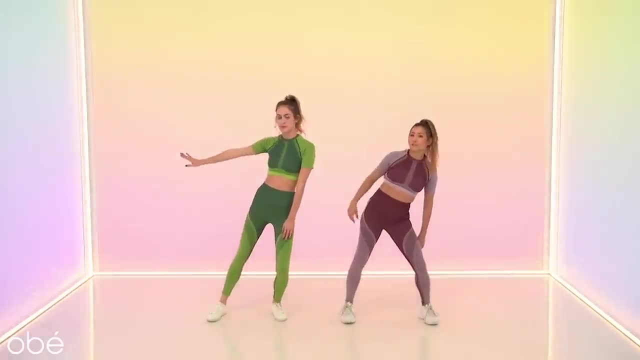 Then you extra three, Four, So you linger on the left. that second time I kinda like the whole body undulation. Hey, ya, That's it. Yeah, just do it. One, Two, Three, Four. You're leaning on that, right. 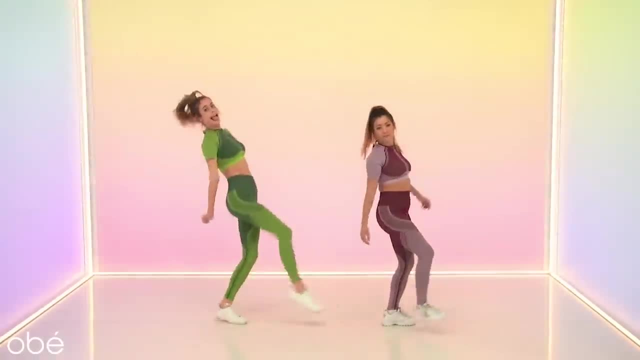 So you're gonna kick with the left. You have to make that noise. So the key to this, if you've never done this before, is you gotta lean back, and then what we're gonna do is, if you're holding two heavy grocery, 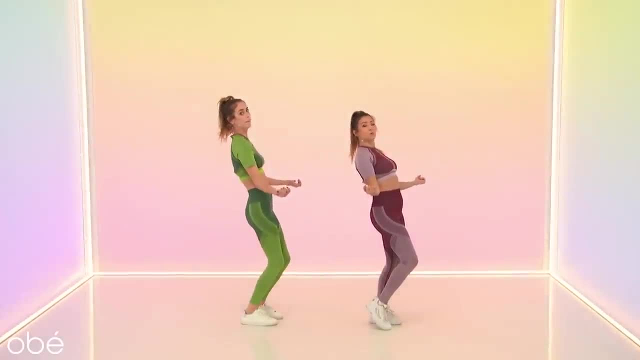 bags. and then you're like, oh no, who's gonna open the door for me? I am with my foot, That's how you get the door open, But now you gotta hop it. Yeah, so your hands don't actually have to. 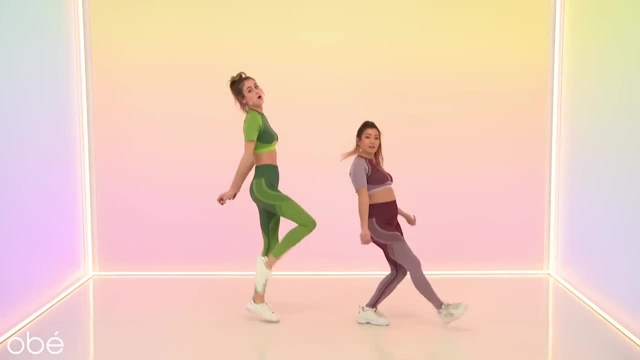 stay here. It just helps you lean back. I've seen people keep them down. If you really wanna go for it, go ahead, knock on the door too. So you have one, Two, Three, Four, Just two, kicks, Five, Six. Now you're gonna. 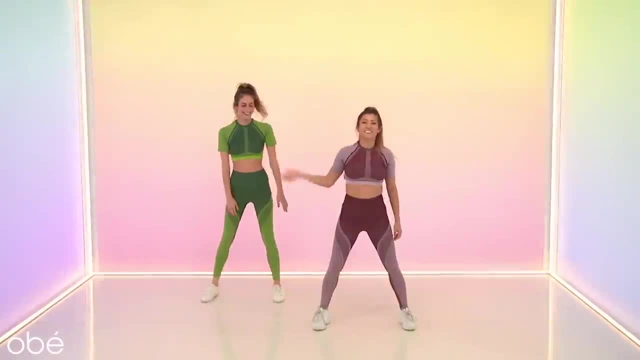 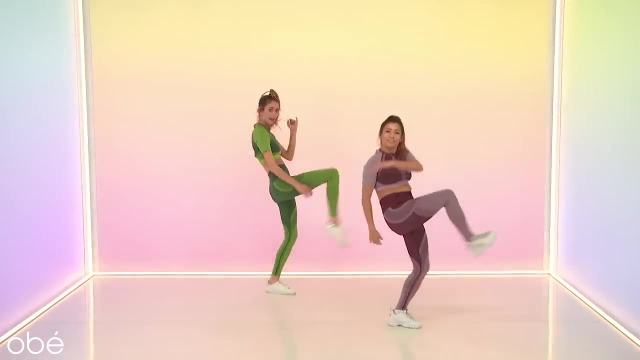 give me big ones: Seven Eight, Five, Six, Seven Eight And one, Two, Three, Two kicks Five, Six Back And front. Five, Six, Seven Eight And one, Two, Three, Kick, Go Five. 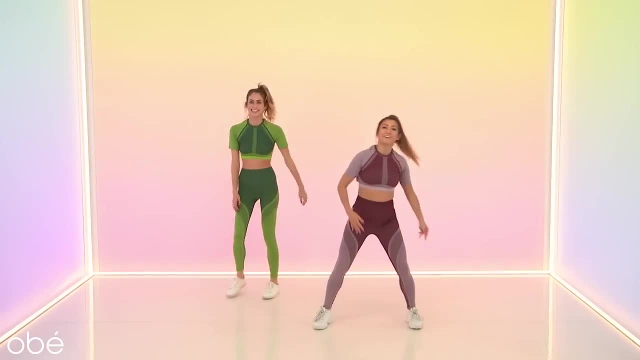 Six And a seven And an eight- It's just faster, You're welcome. Five, Six, Seven, Eight And one, Two, Three, Four And five And six And hop, Hop. So the last thing you just did. 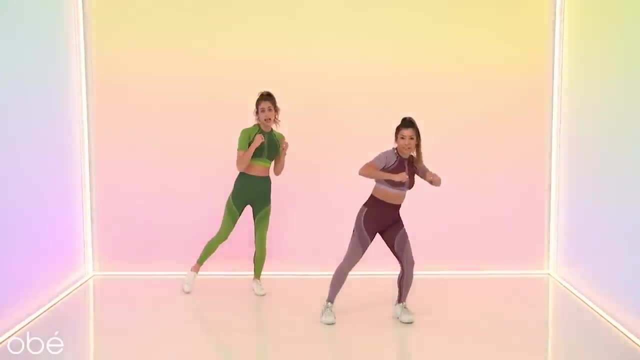 was five And a six And a seven And an eight. So we're gonna swipe it next And one, Two, Three, Step it out, And five And six And seven. Now cocoa butter, Three, Four And kick it. Kick it Then. 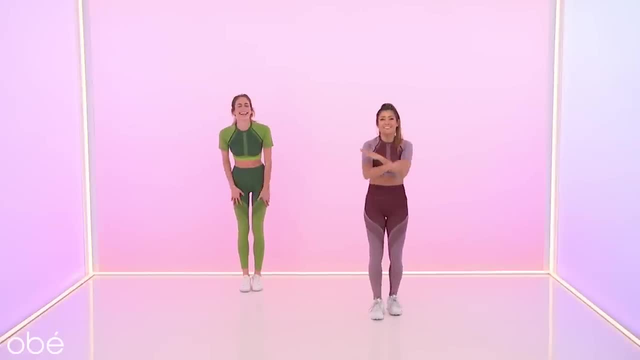 back, Then a front Top it. Here we go: Five, Six, Seven. Left foot goes One, Two, Three, Four Out Five And a six And a seven And an eight. Swipe them One, Two. 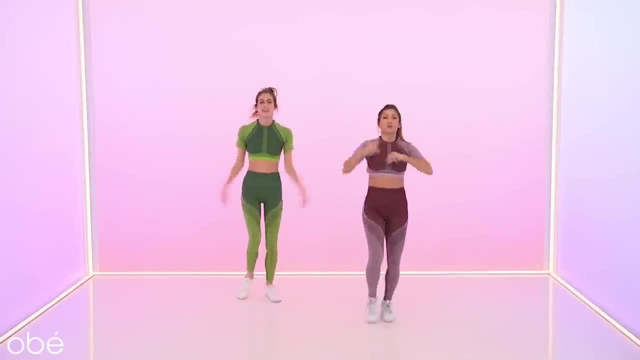 Three, Four And five And six And pizza Cocoa butter One, Two And a three, Four And a five And a six And a seven And an eight, Five, Six, Five, Six, Seven. 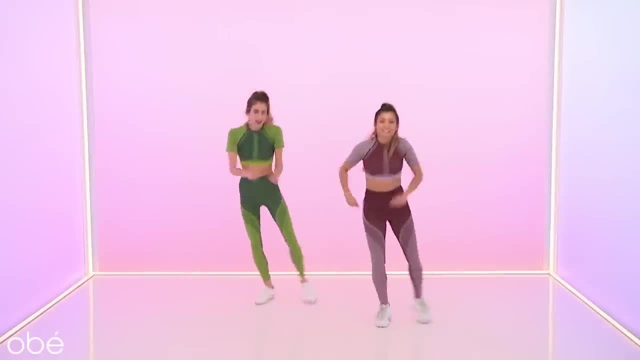 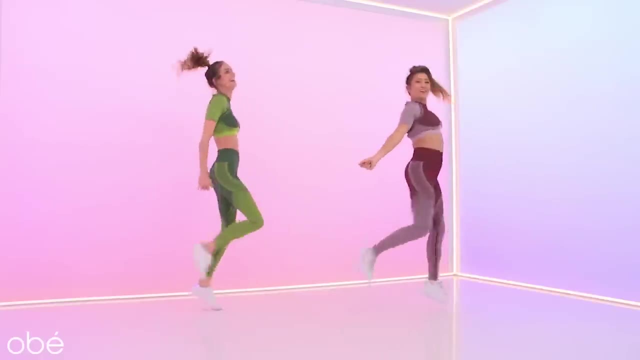 Eight And one, Two, Three, Four And five And a six And a seven. Eight Swipe One, Two, Three, Four And five And six And eight, And cocoa butter Three, Four And five And six, Then kick them. 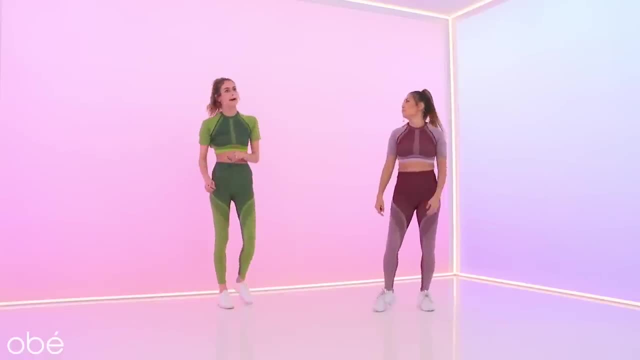 Out. I got a little lost on the cocoa butter part. Oh no, But I'm back. You guys remember Lucy's learning this real time with you. Yeah, So she's going through the same stuff with you. I'm with you, I feel you. 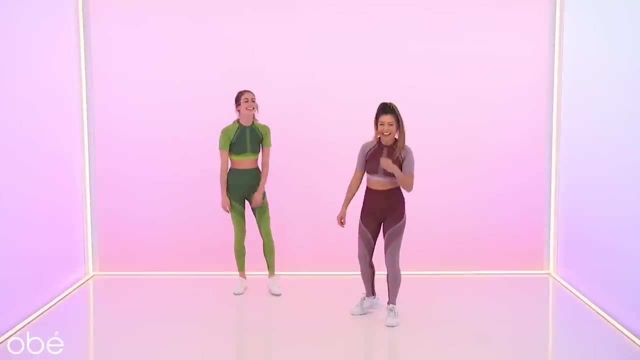 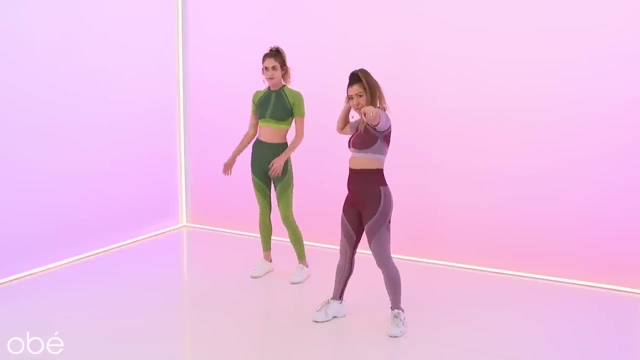 My heart goes out to you. Can we get some music please? Ready Five, Six, Seven, Step it out. Swipe them. Cocoa butter, Let's do it again, please. I see you Ready Eight Out, Swipe them out. 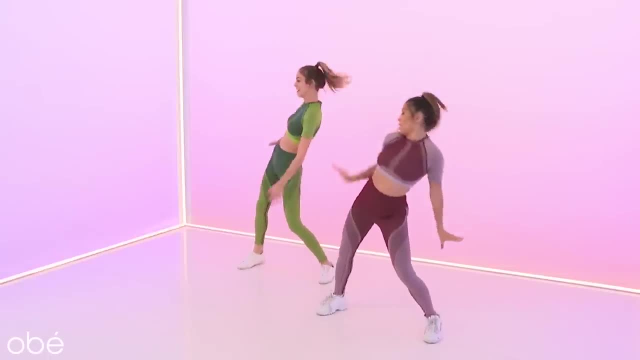 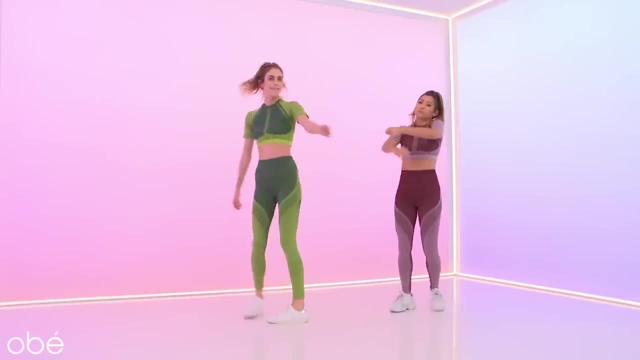 Up Pizza. Cocoa Kick, Kick, Kick. One more time, please. One more One, Two, Three, Four, Five, Six, Seven, Let's go Eight. Swipe them out Up And cocoa butter Good. 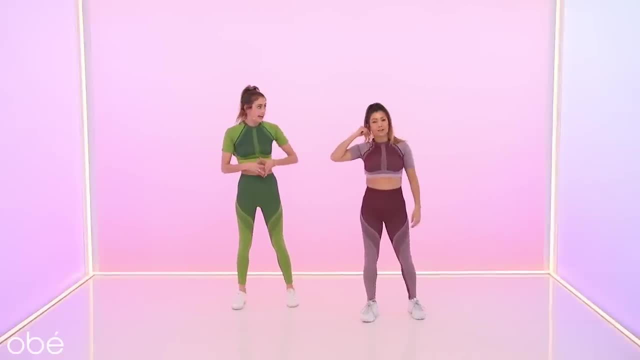 Okay, Good work, We are on the last eight count, The last real eight count. Okay, So you just went five, Six Back Front. So your left is already in front. So you're going to step back with that one One. 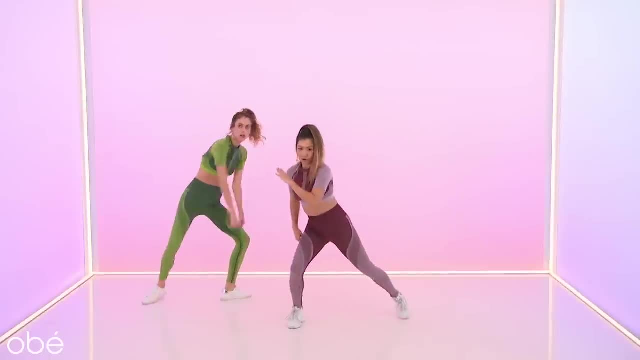 Two, You're going to swing them Three, Four, Five, Six, Seven, Eight, Not bad, Okay, From the foot out, Step, Step, Mm-hmm, Swing her through, Swing. And then you tap it, Then you swing, Swing. 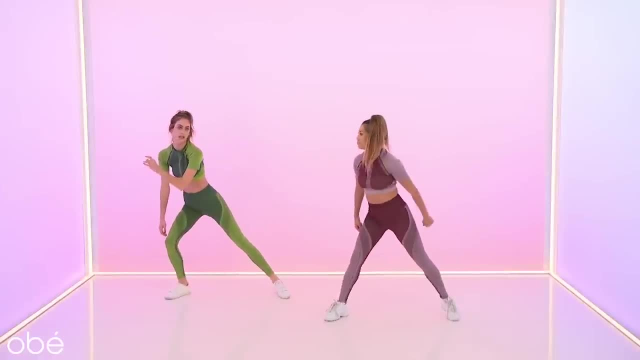 And then you tap it, And then you swing And you tap it. So this is where I'm really going to tell Lucy to drop it low, because I get so low. I know she can do it too, So you just went five. 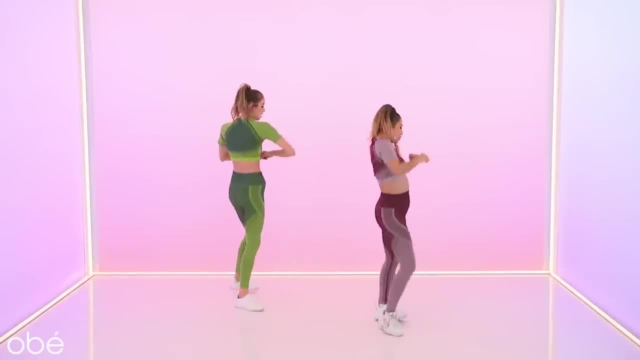 Six, Seven, Eight, Walk it back One, Two, Then swing it, Tap it, Swing it, Tap it, Swing it, Tap it. Now I say, think of a hook pulling your butt up as you're tapping. Oh, I don't know if I can do that. 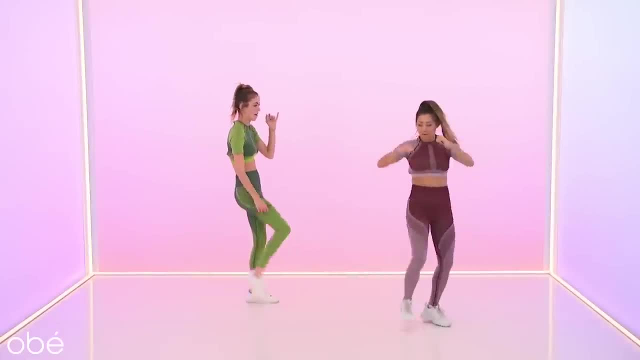 Yes, you can. Five, Six And a seven. Back it up One, Two, Swing them Three, Four, Five, Six, Seven, Eight. One, Two, Three, Four And five And six And a seven. Back her up One, Two. 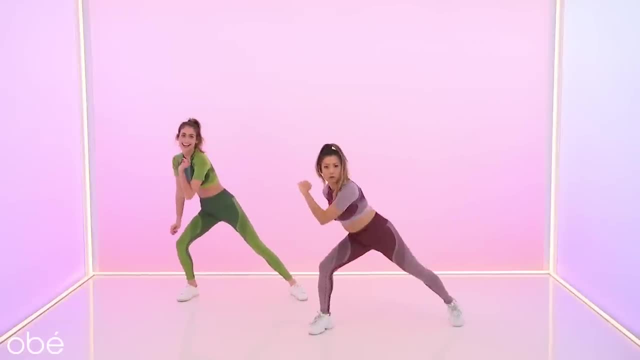 Swing Three, Four, Get lower And get lower. One, Two, Three, Four And five And six And seven. Back it up: One, Two And one And other side And other side. You're done, And this next. 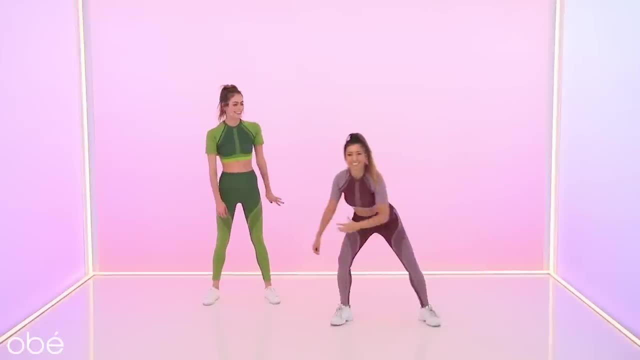 one's like a fake eight. What does that mean? Seven Eight, You're gonna jump out One, Two, Three, Four, Five, Six, Seven Eight. That's it. You get to repeat it The whole eight, Seven Eight, So you're. 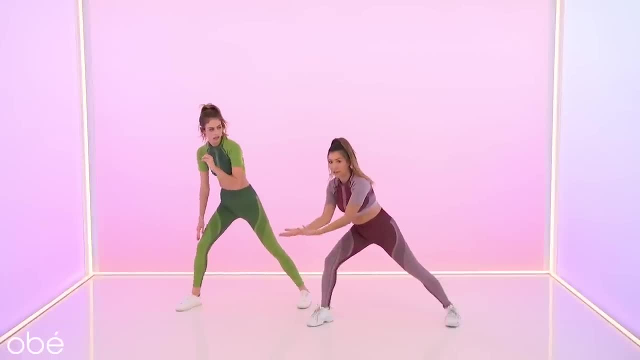 all the way to the left. So I'm not gonna make you jump to the left because you're already there. So I need you to jump to the right. Look at these arms, Then you bring them in. Never hide the goods, Always keep them down. What if the goods? 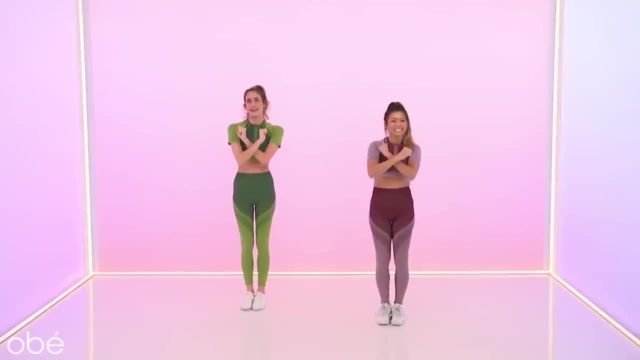 are down here, Wherever the goods are, don't hide them. Don't hide them. Then you go to the other side Again, check those arms, Bring her back, And then you just do it again. Ah, So you have. 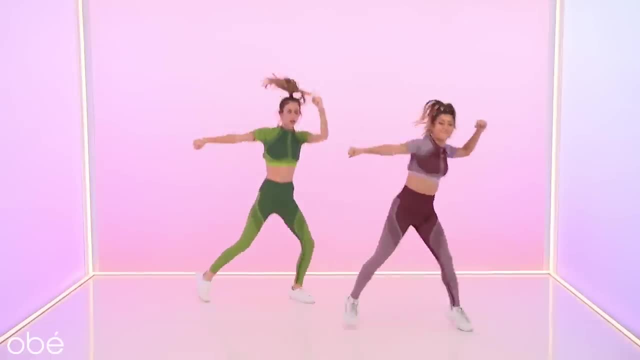 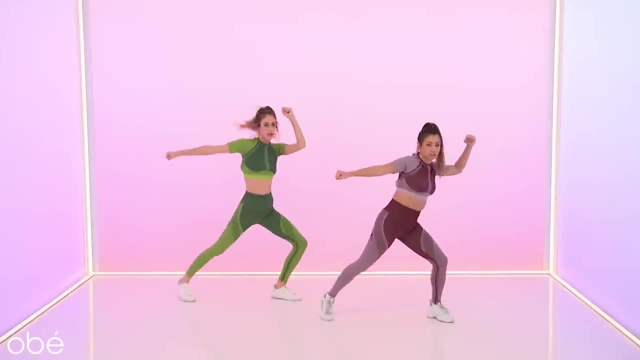 one, Two, Three, Four, Five, Six, Seven, Eight- That's your fake eight. What you're doing is just resetting over your center. You come back to your center. Same thing. You're jumping out over your center. 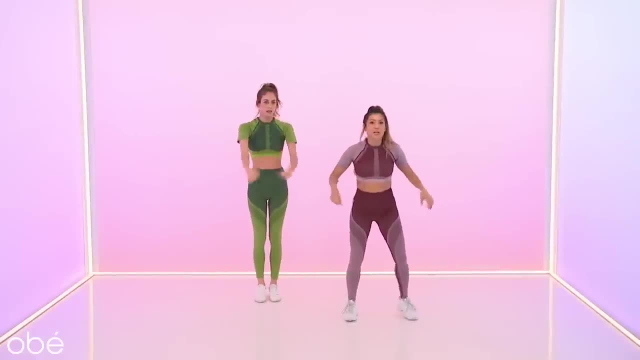 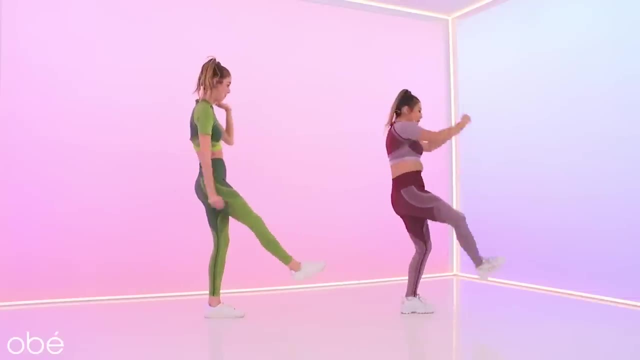 I see There she is, Because if you do the other way, you're gonna give yourself a lot more work and you're gonna be so late. You start over here with a five, Six, Seven, Back her up One, Two, Swing them Three, Four. 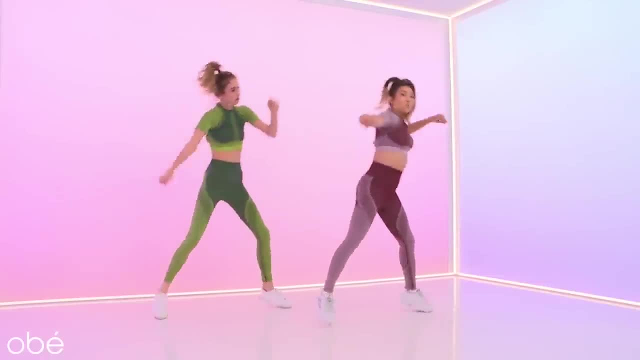 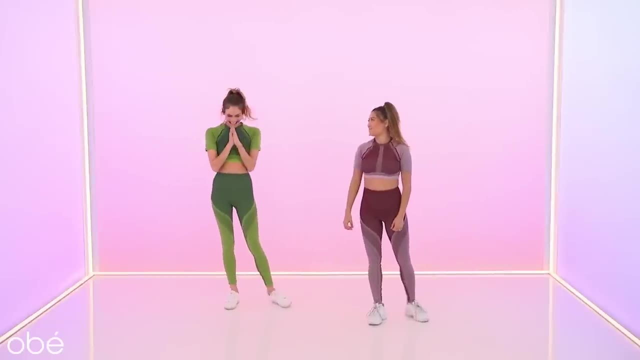 Five, Six. Now you're gonna jump to the right. One, Two, Three, Four, Five, Six, Seven, Eight. Now we have to go back to the top. Okay, Nice and fast, Just kidding, Slow Five. 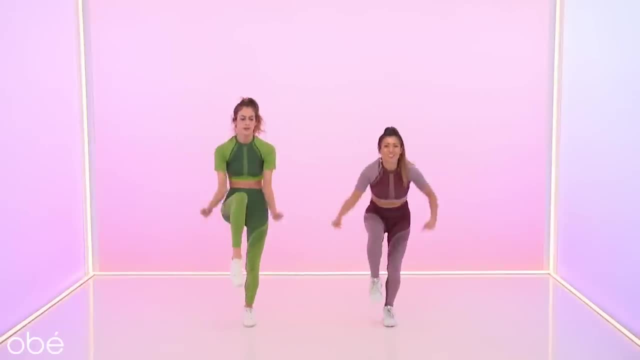 Six, Seven. Step it out. One, Two, Three, Four, Five And a six And a seven. Swipe her out. One, Two, Three, Step it out, And a five And a six And a seven. 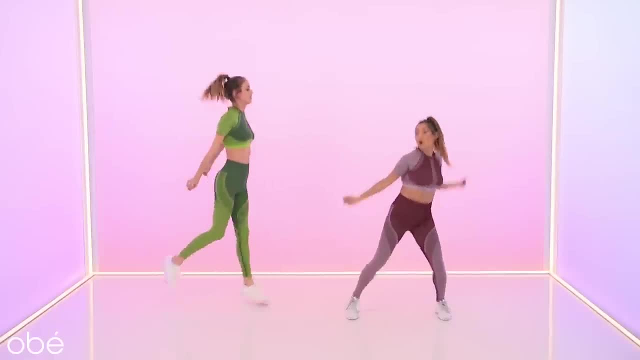 Cocoa butter. One, Two And a three, Four, Five, Six And a seven Back it up. One, Two And a three, Four, Five, Six Jump to the right. One, Two, Three, Four, Five. 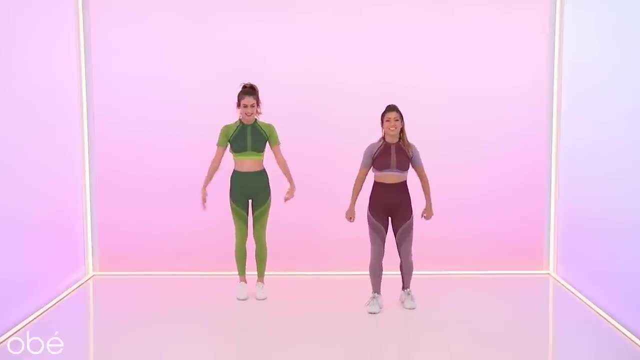 Six, Seven, Woo, Five, Six, Seven. Left foot goes One, Two, Three, Four, Five And a six And swipe it out Next: One, Two, Three, Four And five And six. 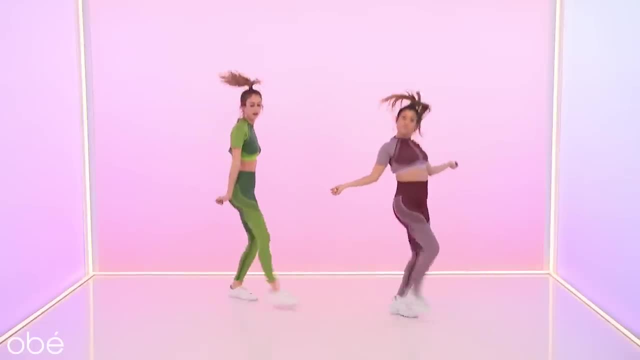 And pizza Cocoa butter. One, Two, Three, Four And five And six And kick them out. Step them One, Two And three, Four And five, Six And let's jump right: One, Two, Three, Four. 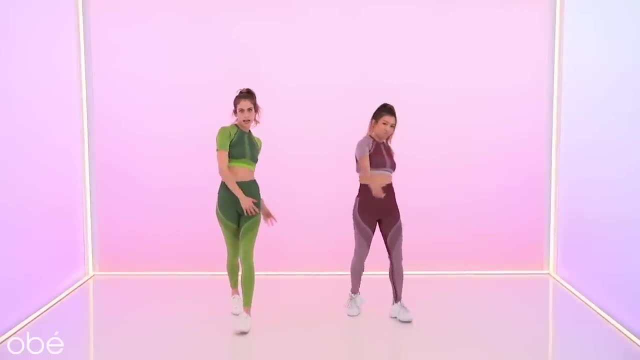 Five, Six, Seven, Woo. Oh, girl, you dance. Oh, you know the words, I like that line: Five, Six, Seven, Eight. And swipe them out, Step them Pizza, Cocoa, Kick them Back it up, And one, Two, Three. 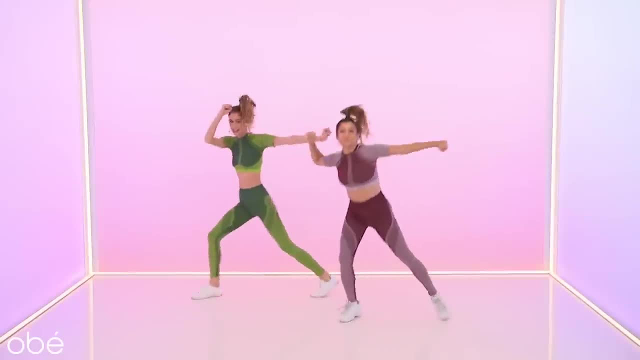 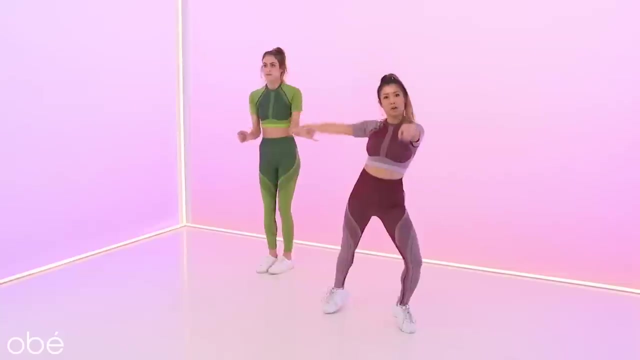 Four And jump it right Again. Yeah, From the top again. Oh, they're still on it. Five, Six, Seven: I'm your biggest fan. Good spin is tuned Cuz I'm into you. Yeah, this. 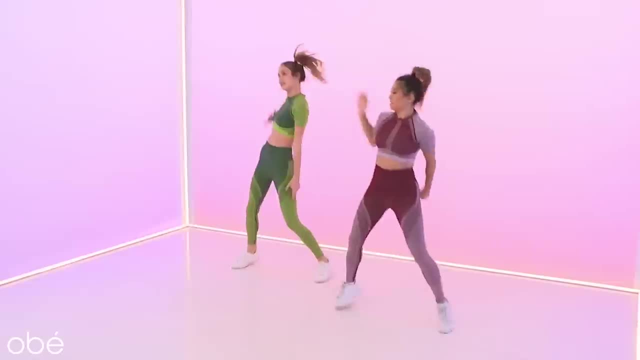 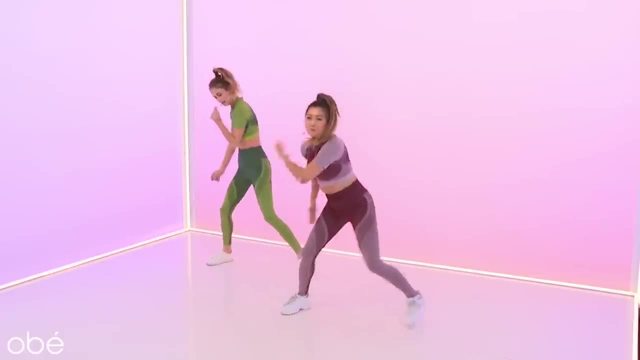 my favorite jam. Yeah, my favorite jam. Everybody lose the crowd. She about to turn it up. She got it up And back it up in planks. Her flow is burnin' out. Jump it right. She starin' in this. 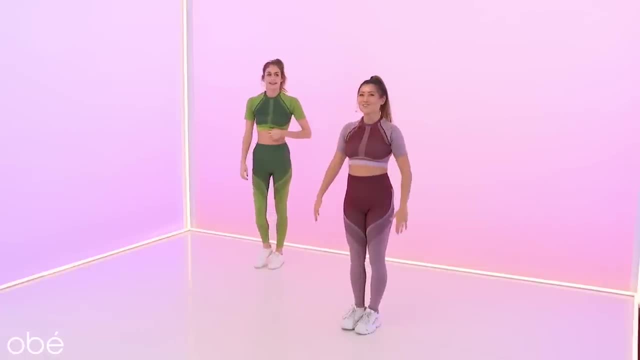 movie And I'm gonna Five, six, seven, hold. Ooh, we're so close to being finished. I'm in love with the DJ. One more time, And I'm gonna count the entire time, just so you have. 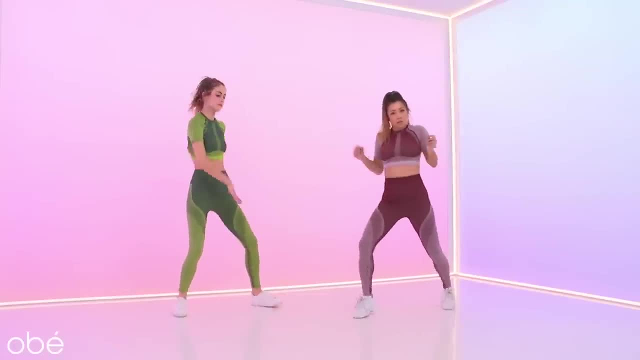 no question. What are the counts? Oh girl, you bad. she hit the track and she shut it down. this beat gonna make you dance. okay, five, six, seven, seven, two, three, four, five and six and seven out and one, two, three, four and five and six and. 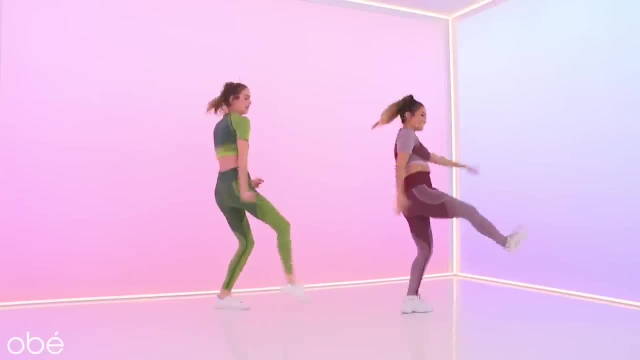 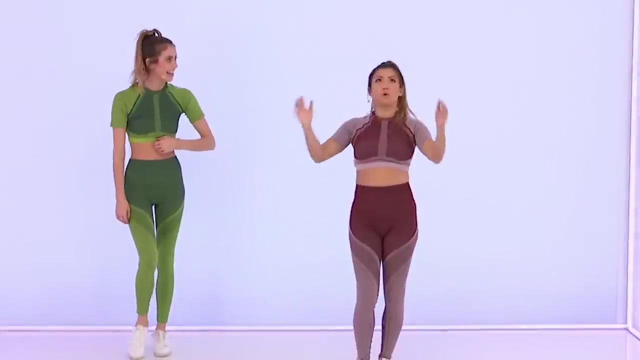 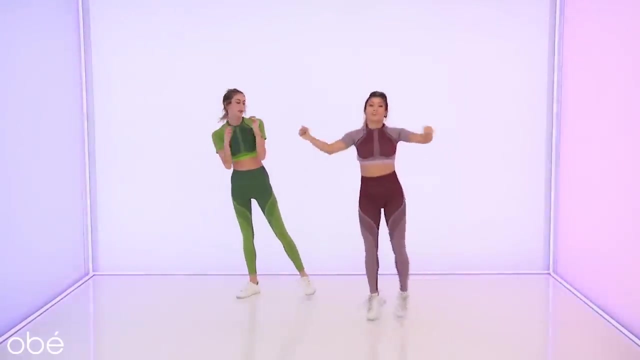 seven, eight. one, two, three, four and five and six and seven. break it up: one, two, three, four, five, six, seven. jumping three, four, five, six, seven, almost done. okay, whoa, this is your outro choreography. we just did one, two, three, four, five, six, seven, eight. you're gonna do the same kind of jump, but go lower, pick up. what should we say? 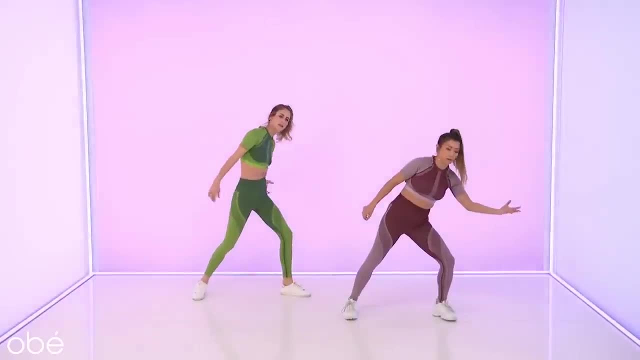 piece of fruit. yeah, pick up a tomato or something and you're gonna throw it across your body onto that wall, onto the left wall. so you're gonna pick it up and throw it. you know a tomato is a fruit. good fruit selection. good fruit selection because i want to see something splatter on that wall. 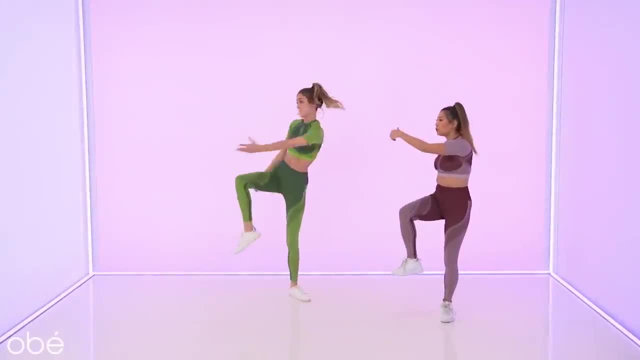 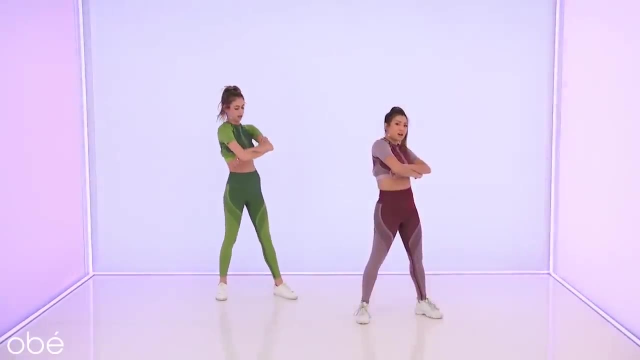 that's how hard you throw it. so you have one. two: you're gonna do it again, but you're gonna throw it over your head. three: you're gonna land four and he goes: i'm in love with the dj and then give us whatever is your favorite move ever: one, two, three, four. then throw the tomato, throw it up. 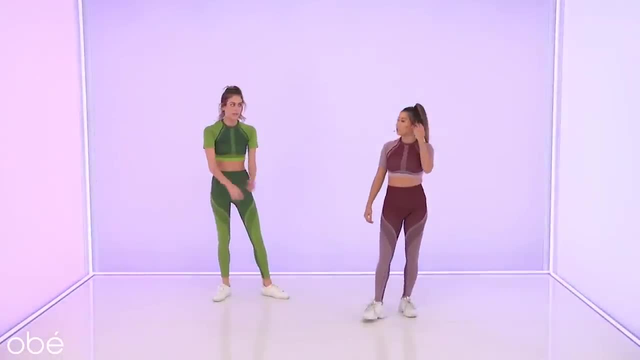 please, okay, oh, and i forgot to land in the cross arm. oh, but you did it. so throw the tomato, throw it up. land, yes, one, two, three, four, hold five, six, seven, oh my god, that's the whole thing, the whole thing. we know the whole thing. even if we can't do it yet, we know it. take it from here. yeah, let's do. 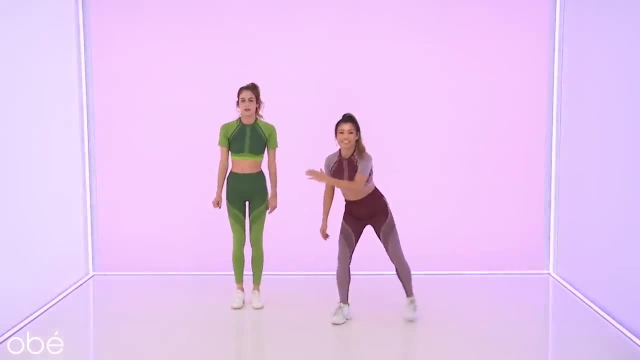 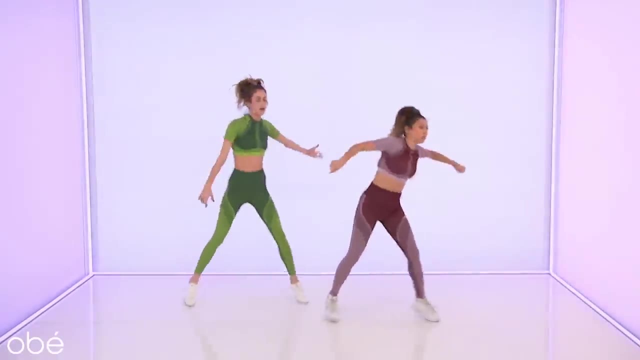 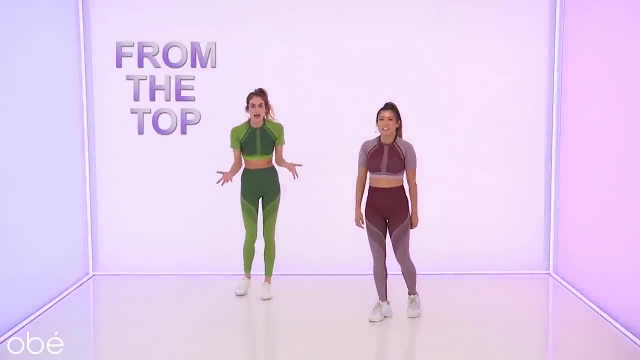 it from here and add those cute little outros on five, six, seven, jump it up and one, two and a three, four and a five, six and seven. here we go, throw it, cross over, hold it six, seven, dj from the beginning. okay, we're just gonna do it: five, six, why not? 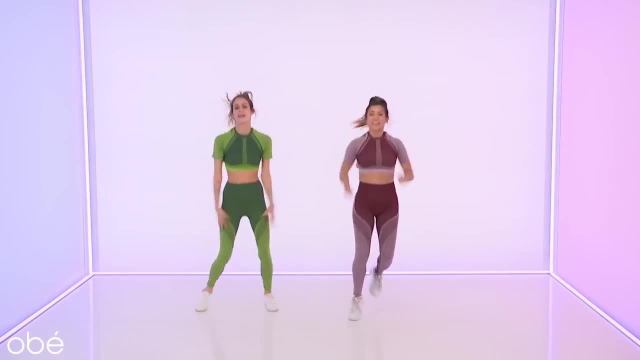 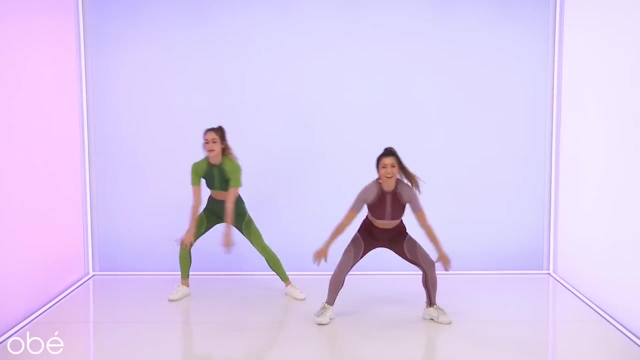 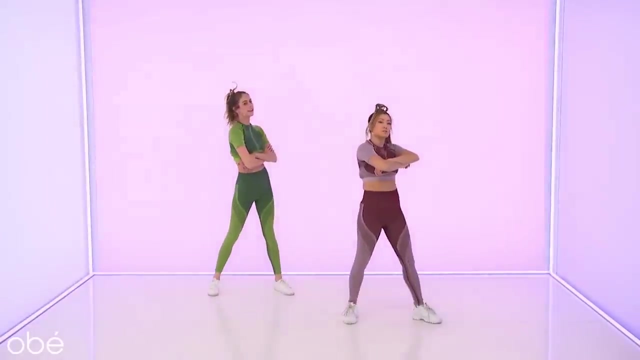 swipe it and cocoa butter goes. kick it, kick it back to the right. here we go: one, two, three, four, five, three, seven. then step across, step it over. hold, i'm in love with the dj, with counts, no music from the top. add everything together and then we're just gonna marathon it. 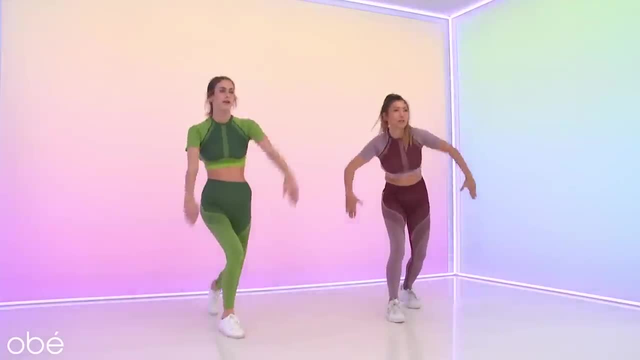 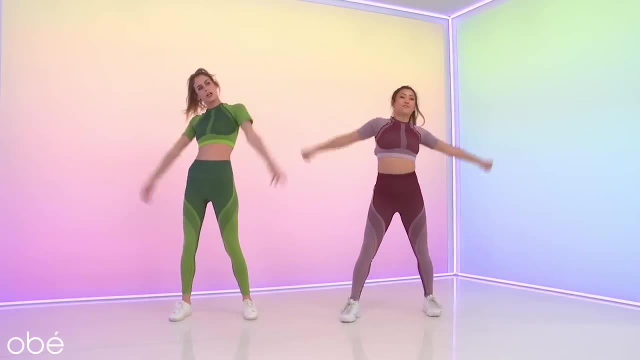 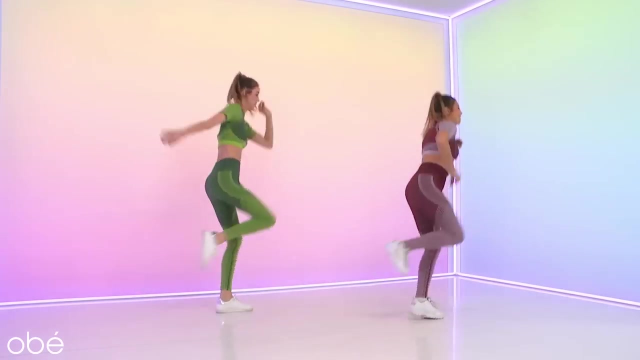 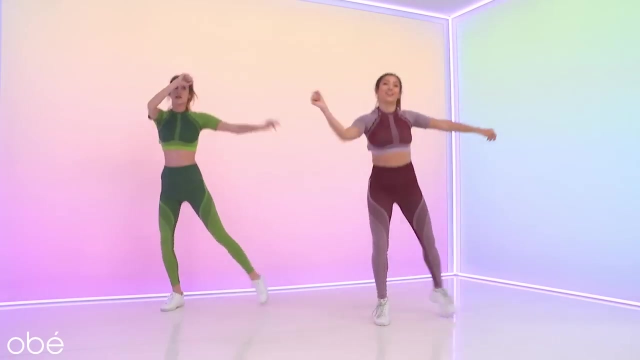 five, six, seven from the top, and one, two, three, four, five and a six and a seven. let's swipe them out: one, two, three, four and five and six and pizza cocoa butter. one, two, three, four and five and six and seven. back it up: left, right, left and other side and other side to the right: one, two, three, four. 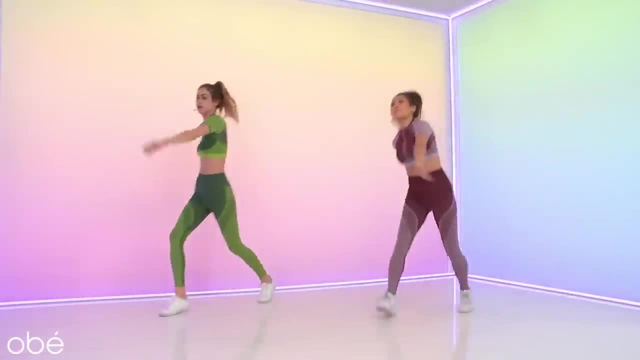 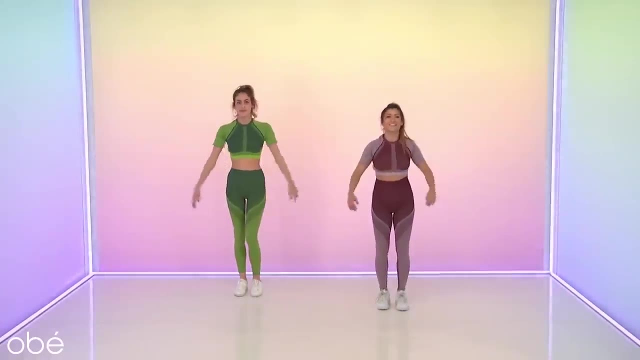 five, six, seven now through the center up above, and five, six. love with the dj. slow again you got it five, six, seven, eight and one, two, three, four, five and a six and seven, eight. swipe one, two, three, step it up and five, six. cocoa butter. go one, two, three, kick them out and five, six back and tuck your back one. 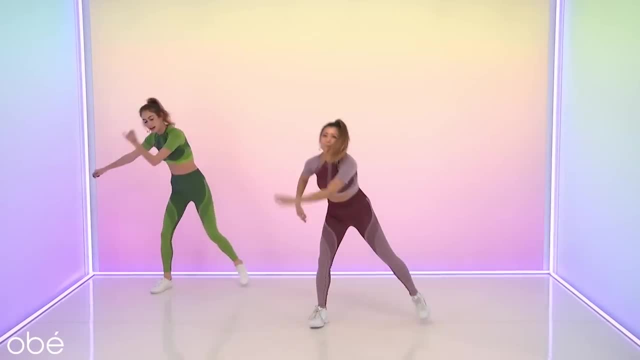 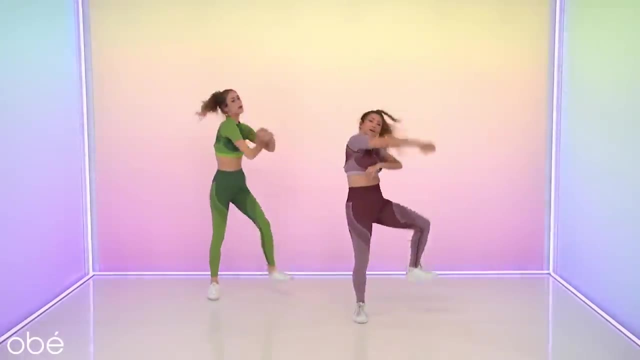 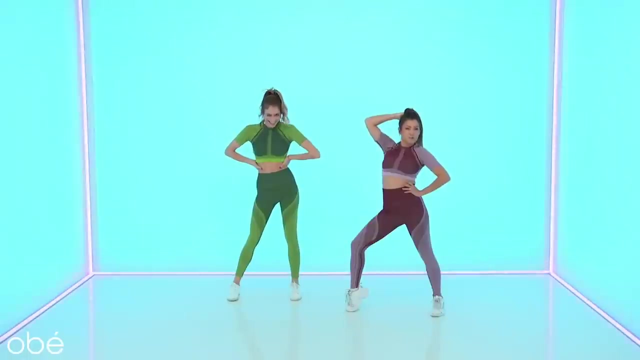 two, swing them and swing them and swing them, jump it out. one, two and three, four and five, six and seven through the center. drop tomato over pause. i'm in love with the dj music. please, all right, let's start with like a cute pose- oh girl, you bet she hit the track- and then move for the face. one, two, three, four, five, six, seven. 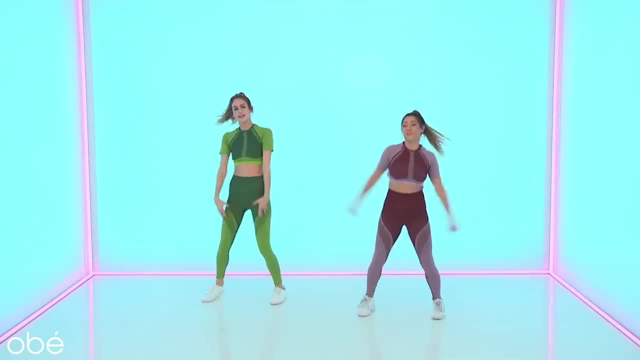 five and six and seven, and one, two, three, four and five and six and seven, eight. one, two, three, four and five and six and seven. back it up: one, two, three, four, five, six in the and one, two, three, four, five, six- nice, swing it in the water jumping out- and one, two, three.